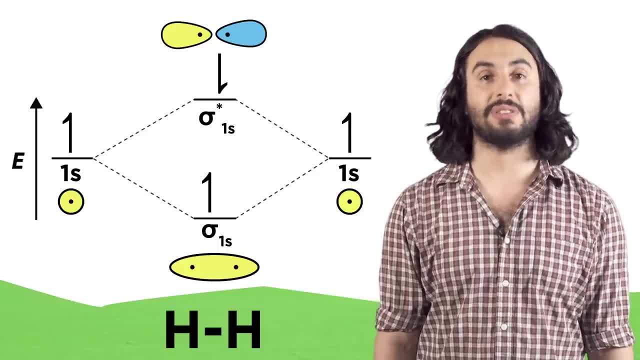 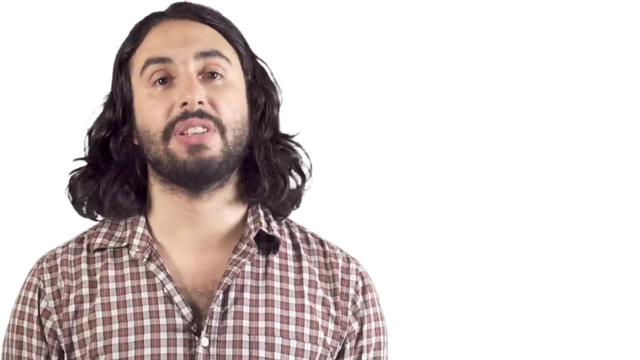 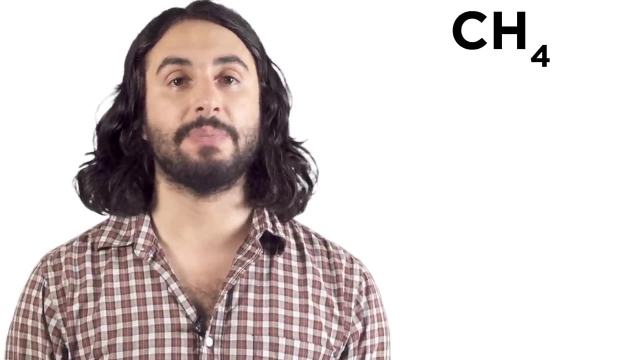 jump from the sigma or bonding orbital to the sigma star or anti-bonding orbital. this is where hybridization comes into play. if an atom is participating in multiple bonds, it will utilize hybrid orbitals to form them. for example, if carbon is making four bonds, as it tends to do, it will take its 2s orbital and 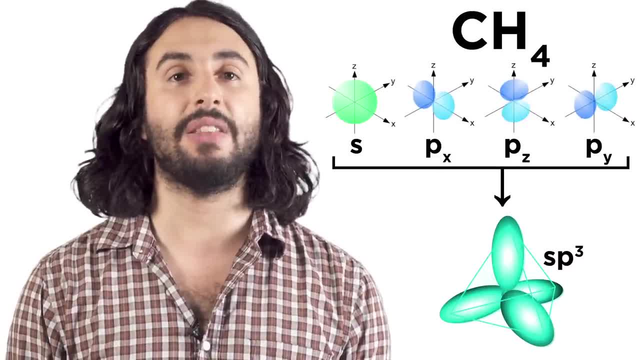 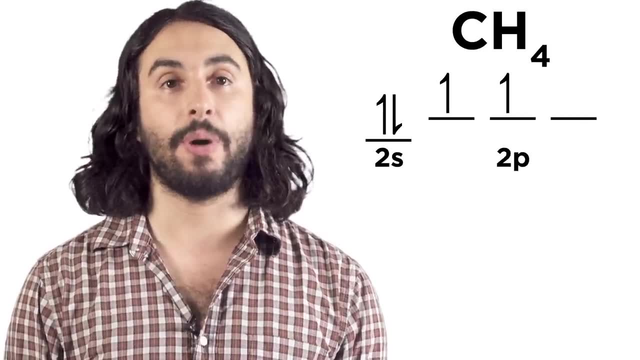 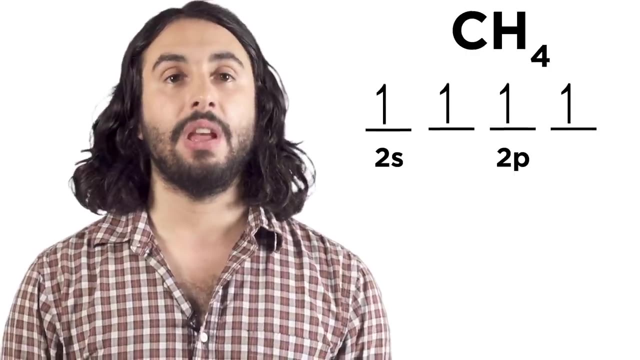 all of its 2p orbitals to create 4 sp3 hybridized molecular orbitals. in order for carbon to hybridize its orbitals, it must first promote one of the 2s electrons up to the vacant 2p orbital. then it can hybridize them, leaving four. 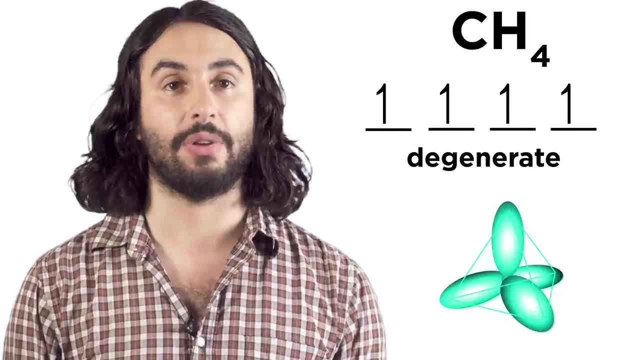 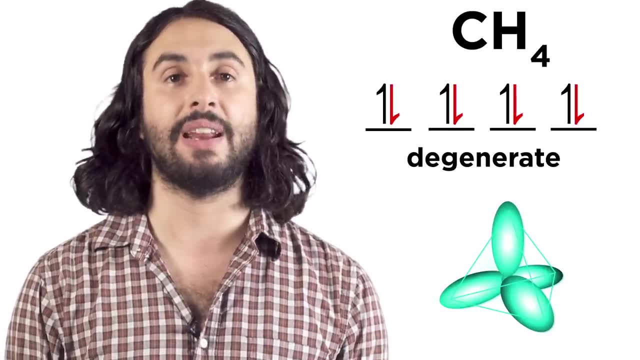 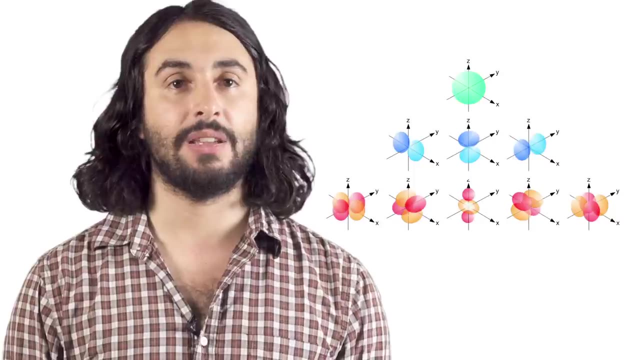 molecular orbitals that are identical in energy or degenerate. each of them has one electron leaving room for another that will be provided by the other atom participating in covalent bond. every energy level has one s orbital, three p's and five d's, and the 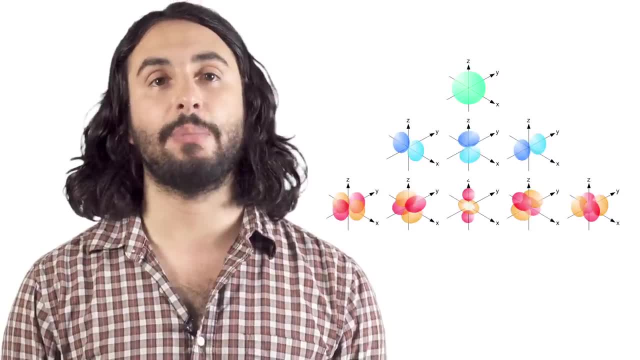 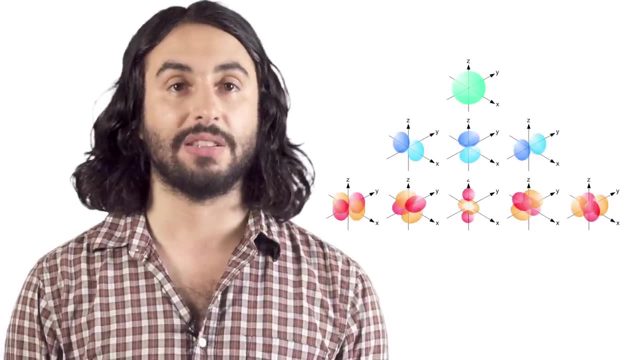 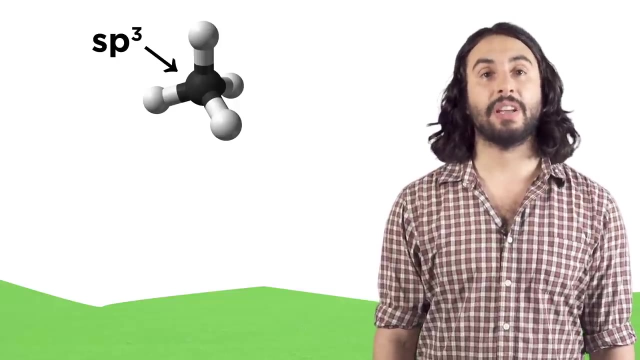 number of bonds an atom can participate in determines the number of atomic orbitals that will need to be hybridized to form the necessary molecular orbitals to generate the bonds. an sp3 hybridized carbon is typically participating in four sigma bonds, but carbon can also be sp2 or sp hybridized. let's look at. 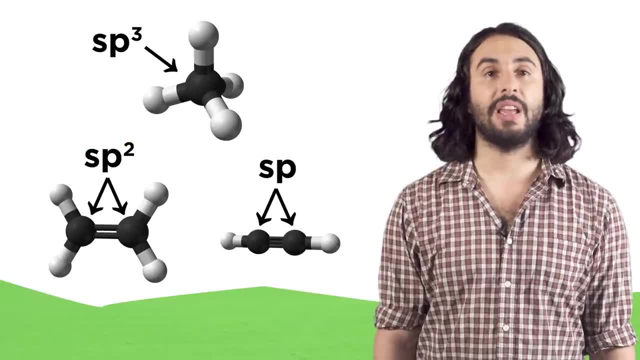 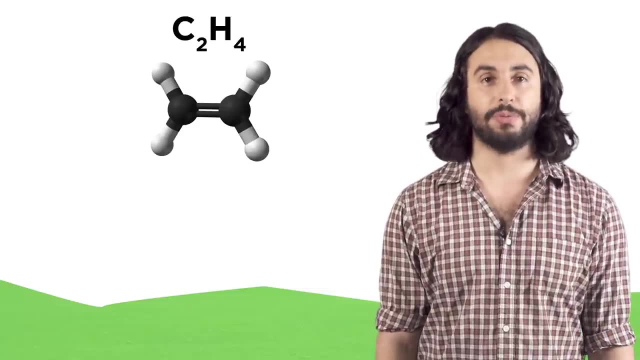 an sp2 carbon. if it is sp2 hybridized, it has just three electron domains, which can happen if it has a double bond to something. take C2H4, for example. each of these carbons is sp2 hybridized because of the double bond present. what this? 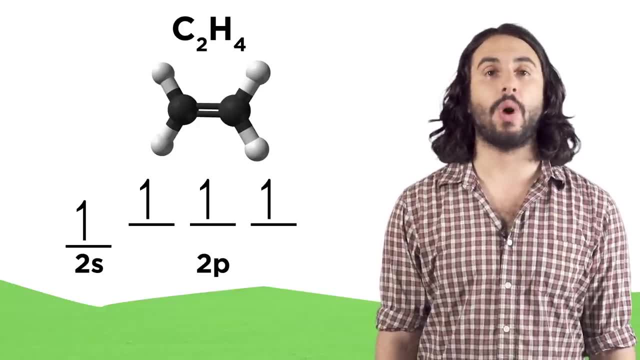 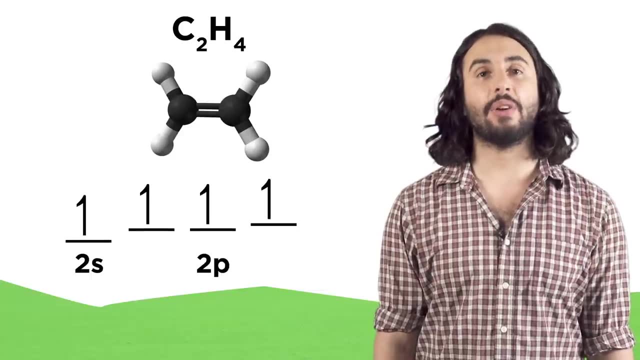 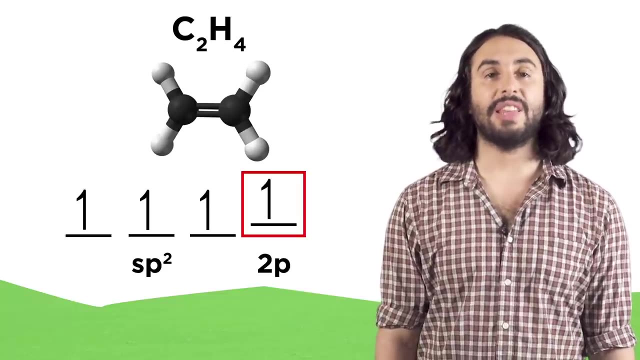 means for molecular orbitals is that the carbon will promote one electron and then take its 2s orbital and just two of the two p orbitals to generate the sp2 hybridized orbitals. that leaves one p orbital unhybridized. it is the overlap of these unhybridized 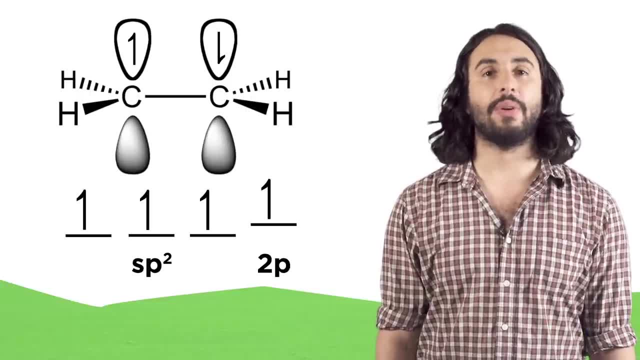 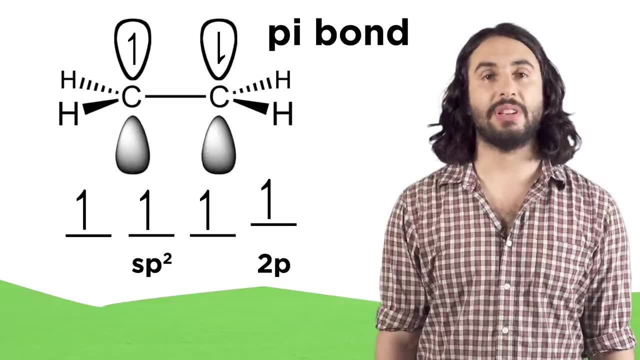 p orbitals each containing one electron. that generates a pi bond, which is what the second bond in this double bond is. the p orbitals extend in perpendicular fashion from the plane of the molecule and they overlap to make the pi bond the. 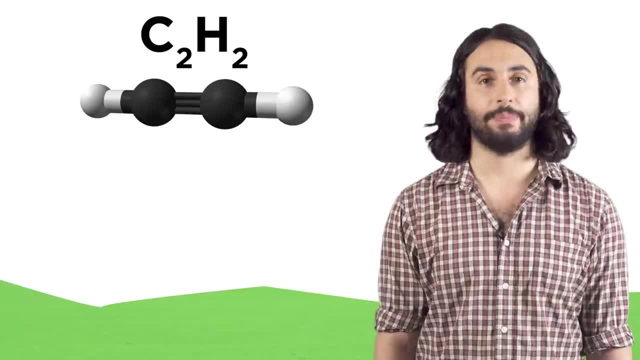 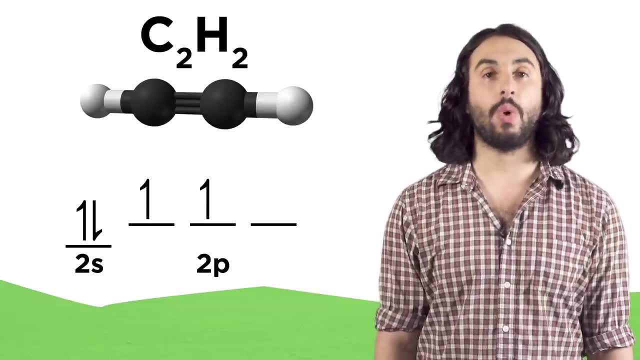 same goes for C2H2,, which has a triple bond between the carbons. each carbon has two electron domains, which means it will be sp hybridized after promoting one electron. it needs to only utilize the 2s orbital and one 2p orbital to get the 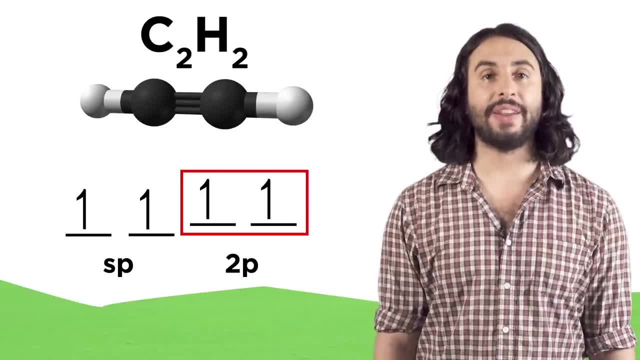 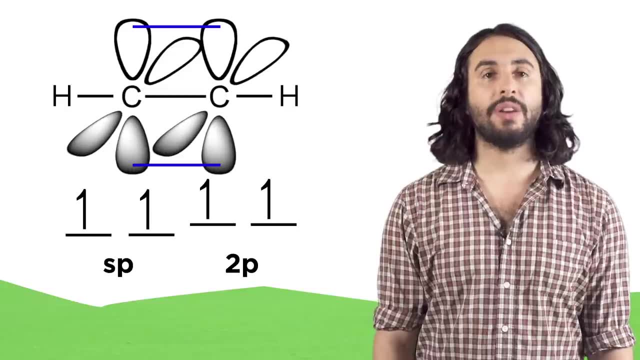 sp hybridized orbitals. that leaves two unhybridized p orbitals, each with one electron. in this case, they will generate two pi bonds, one from the overlap of these p orbitals and another one from the other set of p orbitals that will 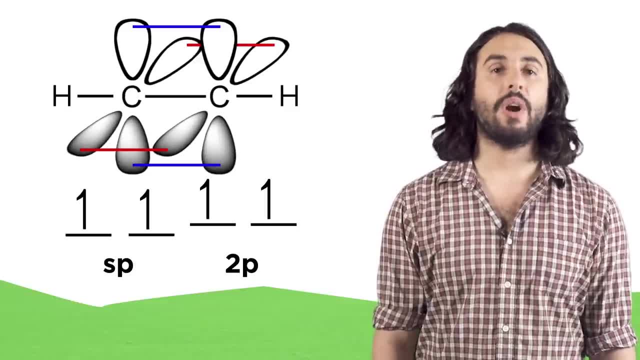 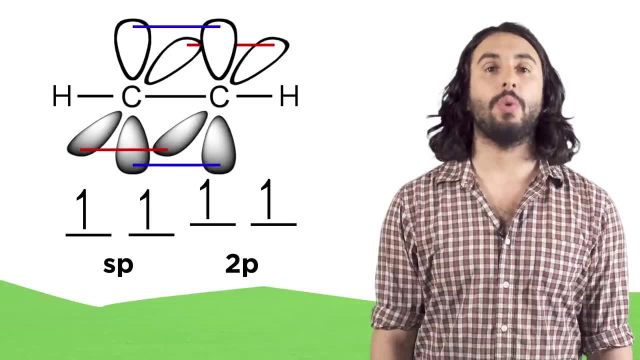 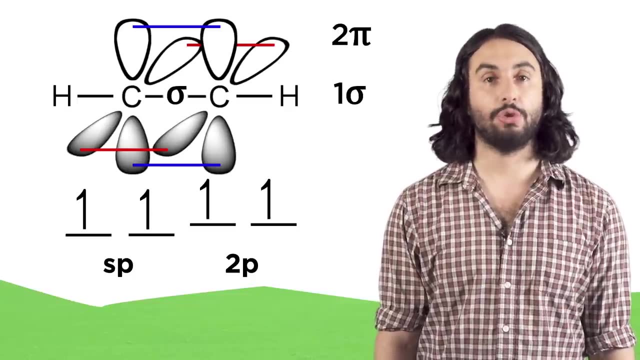 extend perpendicularly from the first p orbital. what you end up with is a linear molecule with this propeller-like orientation of the unhybridized p orbitals, which form two pi bonds beyond the initial sigma bond which is the overlap of the sp orbitals: triple bond: 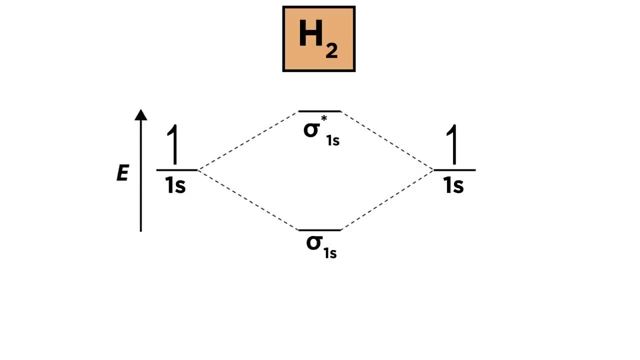 sometimes we have to generate orbital diagrams for a molecule. to do this, we show each atom on the sides with its respective atomic orbitals, and the molecular orbitals go in between. here each hydrogen has one electron in the 1s orbital, so they both go to fill up the 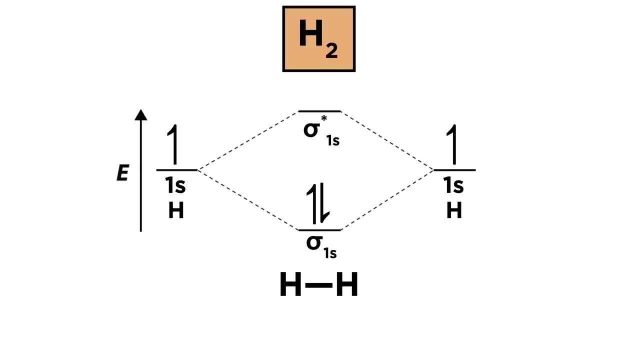 bonding orbital generating a molecule of H2.. we can use these diagrams to calculate the bond order of the molecule, which is given by the number of electrons in bonding orbitals minus the number of electrons in antibonding orbitals, divided by two. here, that gives us a bond order of one, which is why H2. 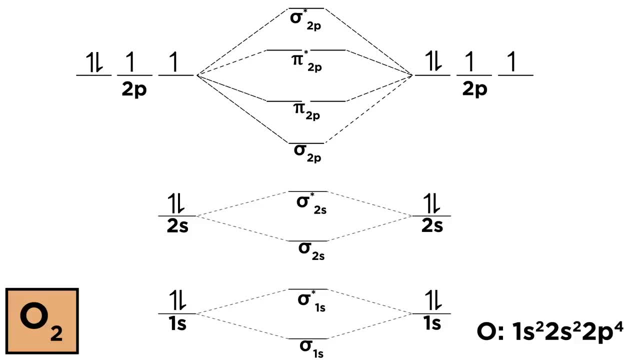 has a single covalent bond. now look at O2.. each atom displays its electron configuration and every electron will go into a molecular orbital. there's the 1s atomic orbitals, which are both full, that go to make the 1s sigma and 1s sigma star, which are 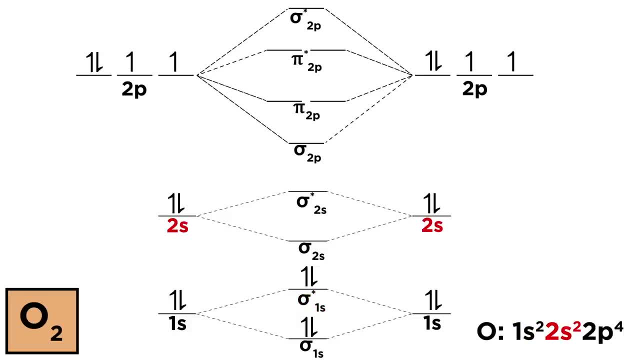 also both full. then the 2s orbitals, also both full, which go to make the 2s sigma and 2s sigma star, again both full. next we have the two p orbitals. each oxygen atom has four 2p electrons. there are six 2p orbitals, total three.